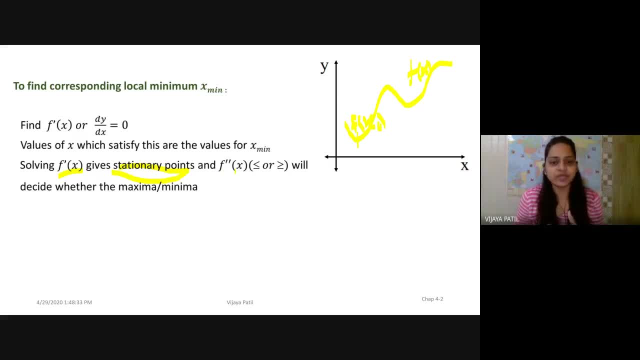 known as the stationary points. then my F double dash of X, whether it's less than or greater than, equals to zero. it will decide my maximum or minimum of this function. what it is, this is nothing but deserve nothing but the stationary points of f, of X, and we are solving dy by dx, 0 for X to find out the stationary. 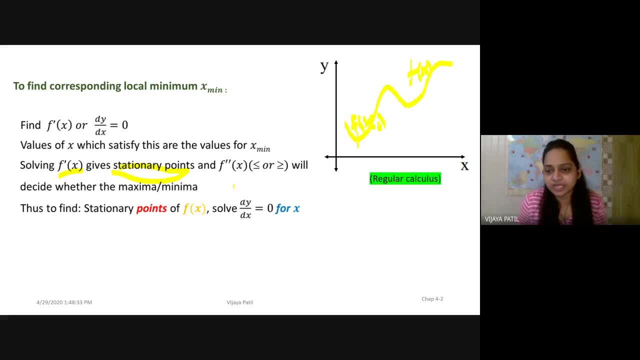 points from this function. this is nothing, but it's known as the regular calculus. what we are doing every time a function is given, we are finding out the local minima and maxima. after this, now let us discuss about stationary functions of functional I of Y. what is this? functional means. functional means the. 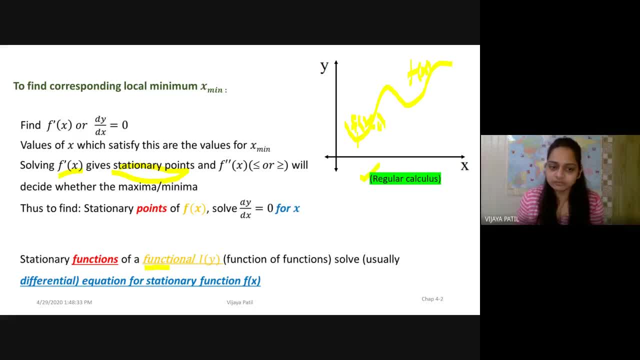 function of functions, right to solve usually differentiable equation for stationary function f of X. now, if we'll compare these two like, this is a regular calculus and what I have defined right now it's nothing but calculus of variations. so we are defining the calculus of variation variations. we are defining those. 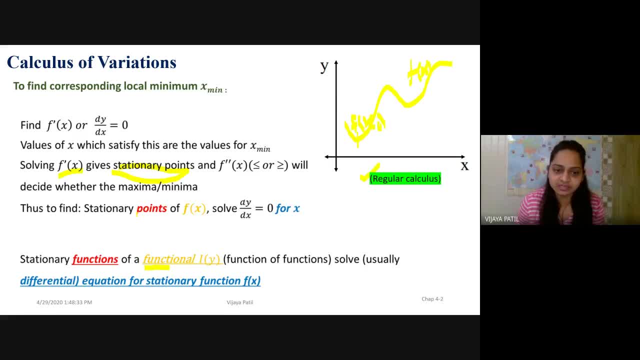 variations based on the functions. so, if you'll observe, I have highlighted these points here, so stationary points. so I have, whenever I'm talking about my regular points, I have highlighted these points here, so stationary points. so I have, whenever I'm talking about my regular calculus, the points regular, the mapping of regular calculus and the calculus of. 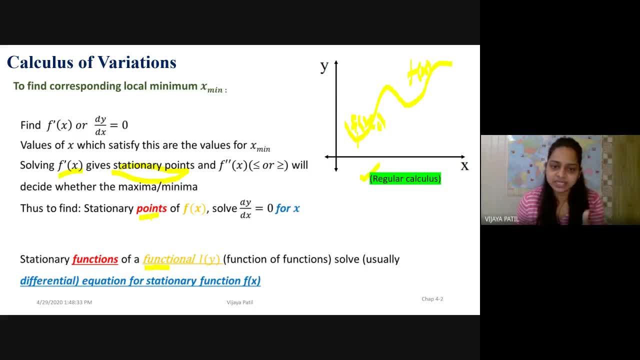 variation if you wanted to have. that is nothing but in the calculus I have a points in the calculus of variations, I have the functions, if it is of f, of X, here, for what I'm finding out, the stationary point, here they are functional. functional is nothing but a function of functions and this is what 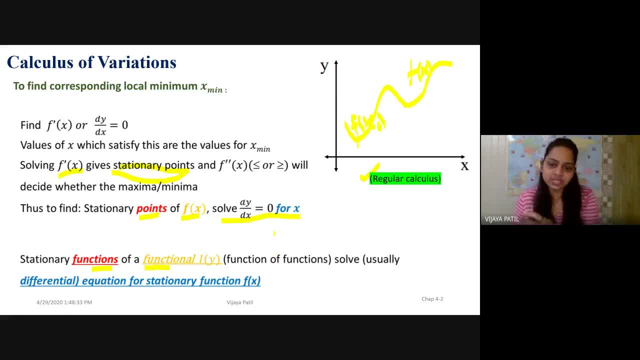 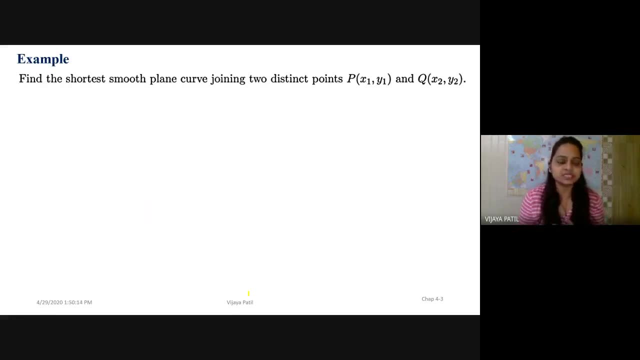 the differential equation- we are doing it here right now in the regular calculus that is been that role- has been replaced by the differential equation for stationary functions of f, of X. okay, let me just give you the more explanation are with the help of example. now suppose my example is find the shortest smooth. 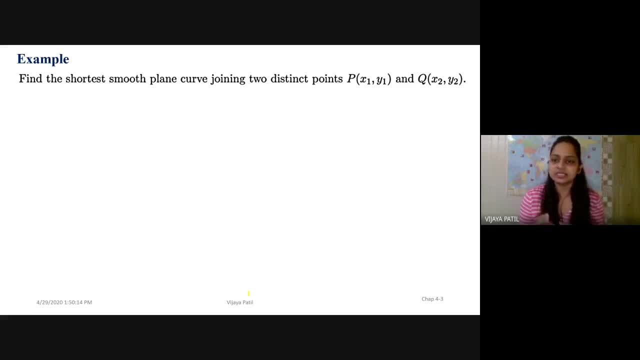 plane curve joining two distinct points, say for P of X 1 comma Y 1 and Q of X, 2 comma Y 2. now, if we observe this, that means what I have got: two points, P and Q, and I wanted to find out a smooth plane curve. and I wanted to find out a smooth. 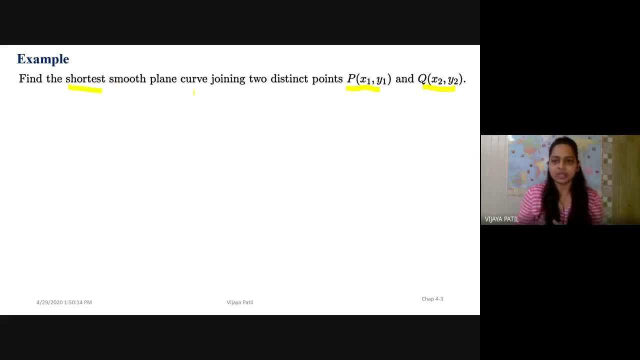 shortest smooth plane curve, and we are aware that by by just two points I could find out: the shortest is the shortest. like shortest curve is nothing but a straight line like this. let us do that. so, if I have got this, P X, 1, Y, 1 here, Q, X. 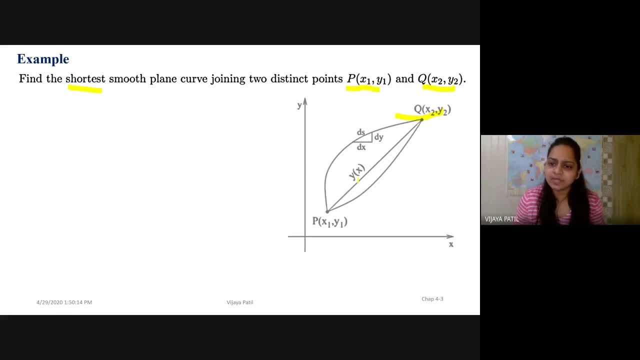 1 Y 1 here, then from this two points I am. I am getting infinitely many curves which can join these two points, but what is my thing, what my constraint here is: I need a shortest. so I need a shortest curve right now. let us consider on any. 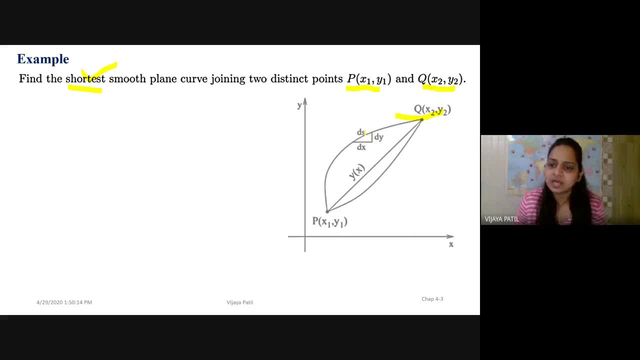 random curve. I am taking this curve and I am considering here this, a small part of this curve. it's known as a DS. right, this DS? what this DS? and if I am, I am putting a perpendicular parallel to Y axis, here, I am putting a perpendicular parallel to X axis. I am getting my dy and DX over here right now. this is what. 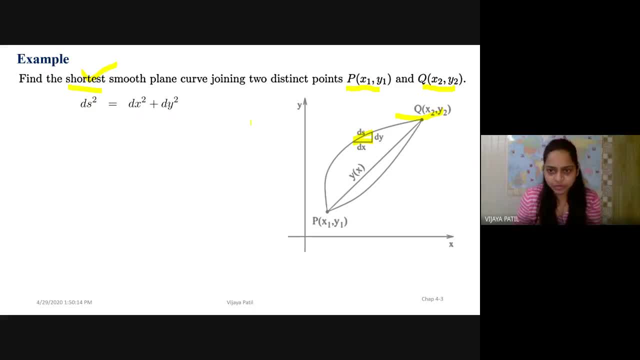 is it? it is nothing but dx, no del x. and if I am trying to write under this: a ds square is dx square plus dy square, that is, by just a right angle triangle law, then this is nothing. but if i'm taking multiplying both the sides by dx square, i'm going to get ds upon dx. 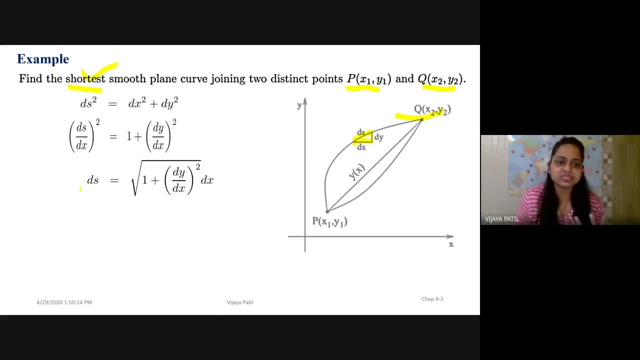 square, this will give me 1 plus this, and which is nothing but ds is equals to square root of 1 plus. so what is it? this is nothing but just a ds. we have written in terms of the dx and dy. so what is it? this is nothing but a total length. total length of this integral p to q, ds. ds is on. 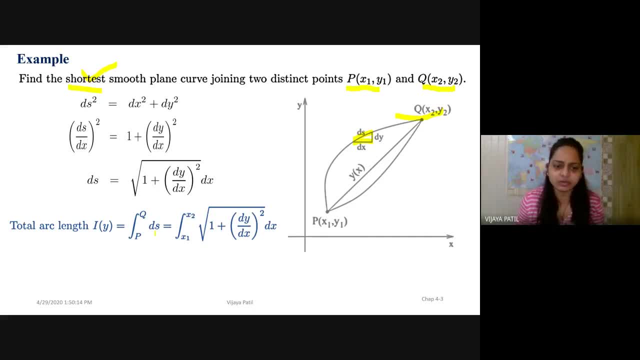 the surface or on the curve. here it's a nothing but a line, integral or integral, which is e. this is equals to integral from x1 to x2, because i'm i'm integrating this integral with respect to x, so my integral, the limits would be for this. so this is x1 to x2, square root of 1 plus dy by dx. 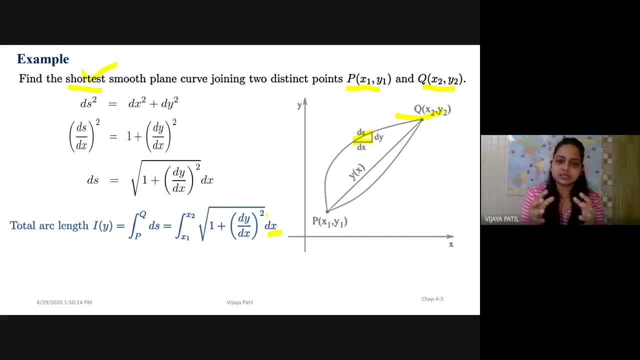 square. so this is an, this is a, this is a an approach of the question in the variation of calculations, calculus or calculus of variations. both the things are, you can just go ahead. so this problem is getting converted into our calculus of variation as minimize, minimize this. so this is what is what.